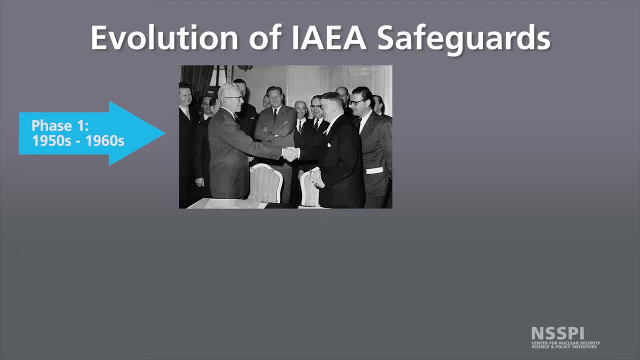 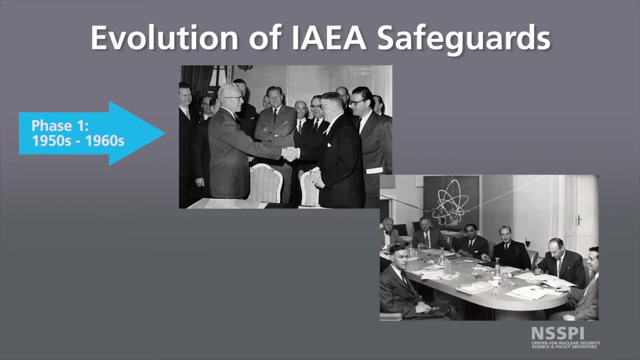 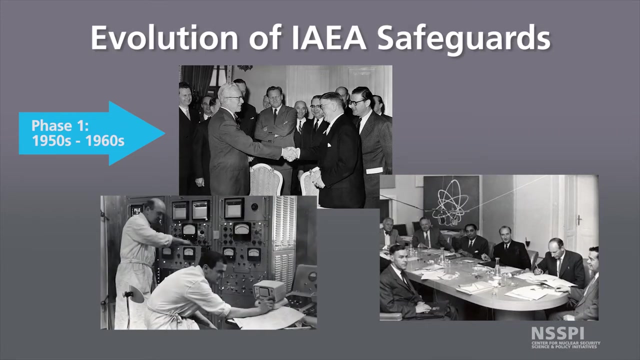 the creation of the IAEA in the 1950s and 60s, as nations were just beginning to trade in nuclear technology and supply nuclear facilities to other nations and trade nuclear fuel. They're just learning how this would occur. The IAEA safeguards system is established to ensure. 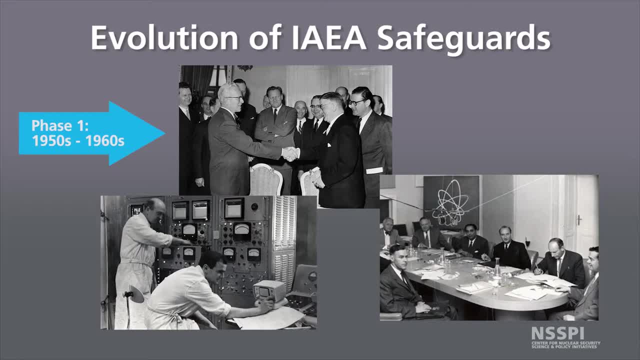 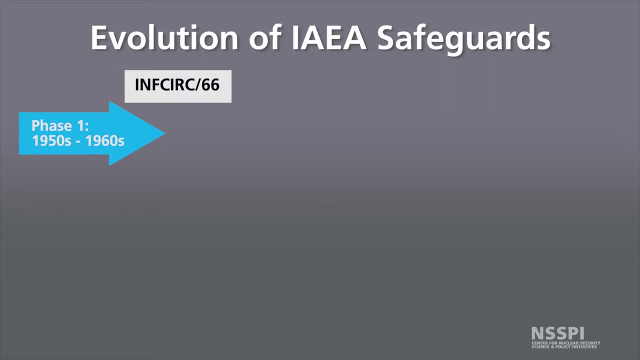 that this did not lead to the spread of nuclear weapons And this is encoded in instances of the 1960s and 60s. So the first one is the Infocerc 66, which, spelled out, refers to information circular which is an approved document from either the UN or the IAEA. also, 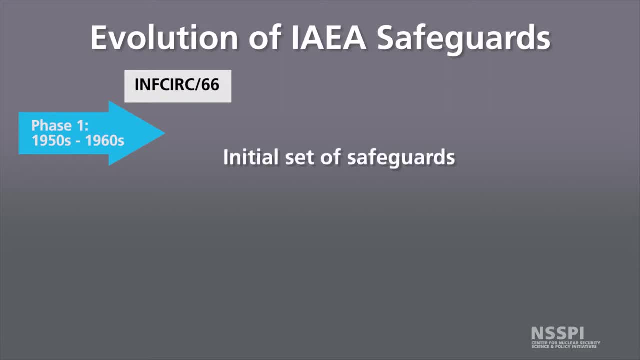 distributes information circulars And Infocerc 66 was the initial set of safeguards that the IAEA would use to safeguard the international nuclear industry About 1991, that begins with when the NPT was signed, the Non-Proliferation Treaty, the 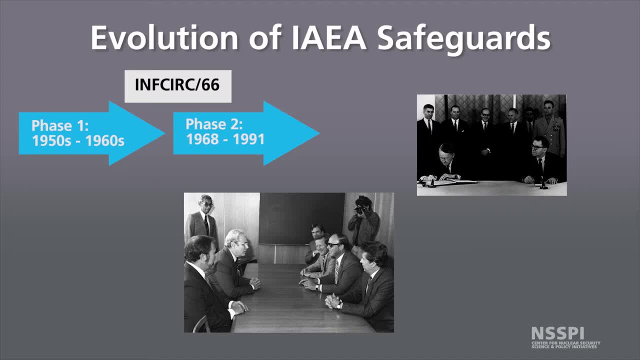 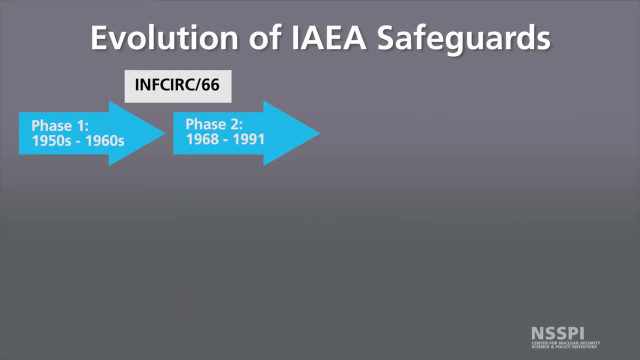 IAEA was legally tasked to apply safeguards on all nuclear materials in non-nuclear weapons states that were party to the NPT. So this expanded the role of IAEA safeguards, before with just Infocerc 66. The IAEA safeguards were applied only where they were agreed to. between the two parts of the IAEA and the United States. And even before that there were no safeguards to apply to all the nuclear materials in non-nuclear weapon states. So this expanded the role of IAEA safeguards. Before with just Infocerc 66, the IAEA safeguards 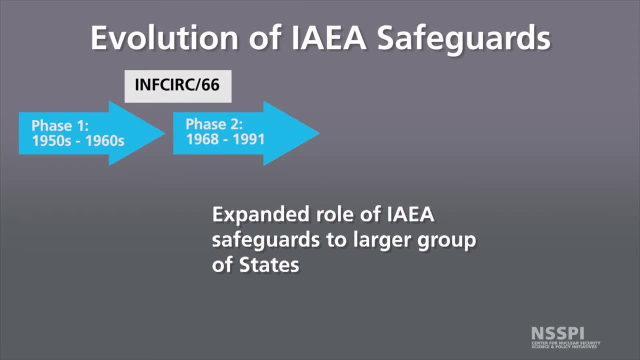 different states and the IAEA, whether that was required by a supplier state or not. There are several scenarios when they could have been implied, But beginning in 1968, when the NPT was negotiated, all non-nuclear weapon member states of the 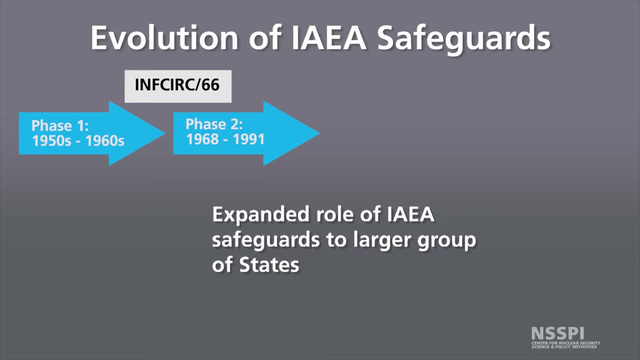 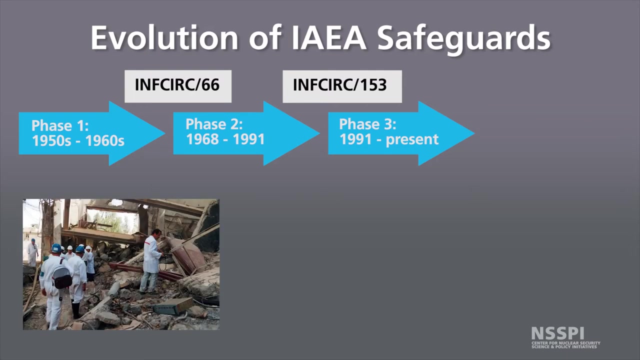 NPT were required to have IAEA safeguards on any nuclear material within their borders, And this is referred to as INFCIRC 153, Information Circular 153.. And then in 1991, there was another revision to the safeguard system. This came about due to the clandestine nuclear weapons program in Iraq and also some of the